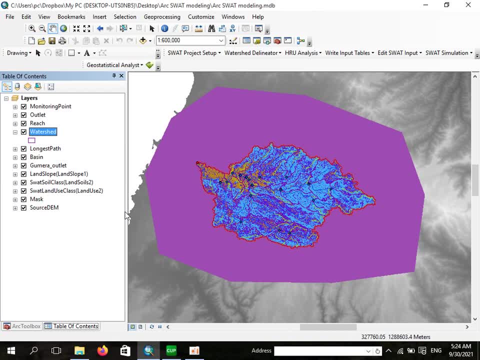 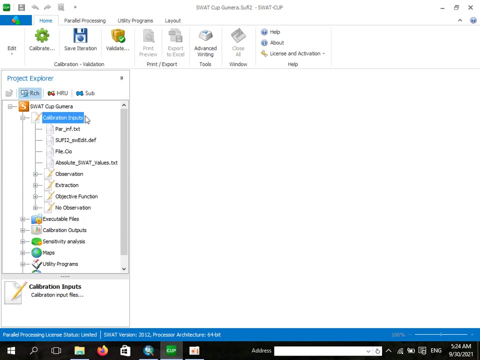 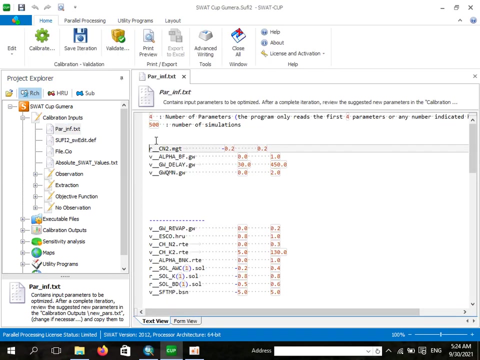 model using a simulated and observed stream flow. in case of stream Flow, therefore, you should have such a date us. so for such purpose, let us start our work here. give you an introduction: in the last video, you should have this parameter information here. you should insert your parameters here, okay, or parameters here: 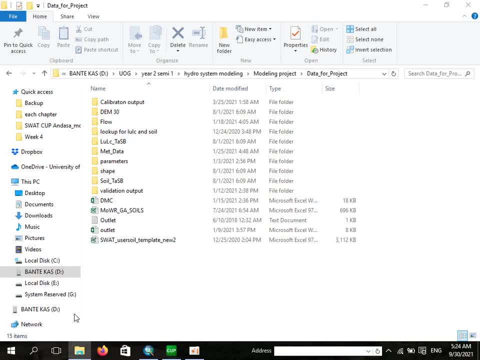 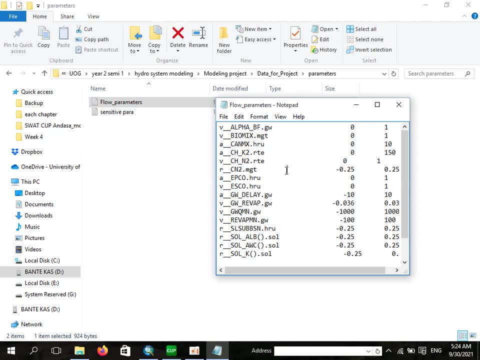 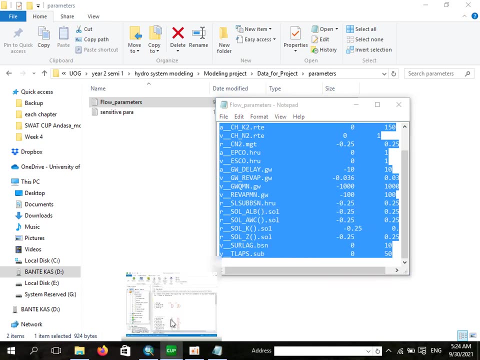 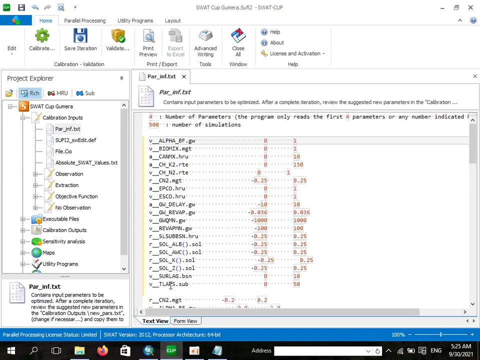 so I have a parameter here: flow parameters. actually these are my parameters. what I have selected, select all. sorry copy. go to SWAT cup here, paste your parameters and I can count it as around 19 parameters, one nine and I would like to do around 20 simulations to reduce the time for. 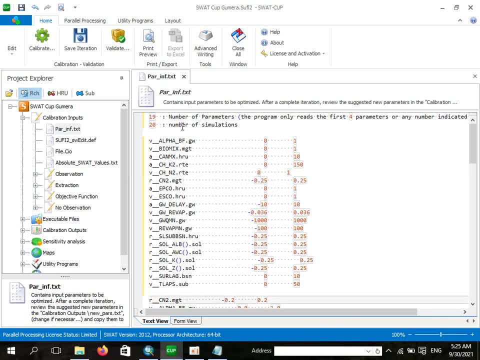 a video or edit one the other video to reduce the time for, or edit one the other video to reduce the time for the work. but you can increase, since this sensitivity analysis to know to identify which parameters are sensitive. so you should at least do a Tony and number of. 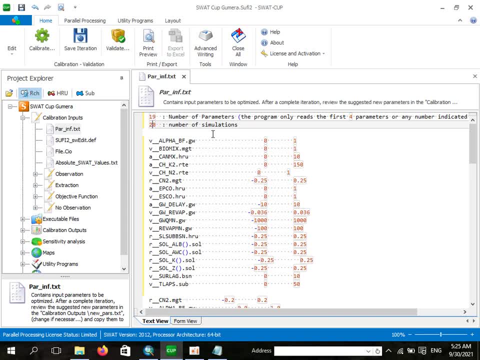 simulations. that is why I am giving Tony okay, so, and for this tutorial. but you can increase your number of simulations more than 20 to get, or to get exact sensitive parameters. so, and let us use this one. so if you count this one, those are 19 numbers, and to check that you should click on form of use and check. 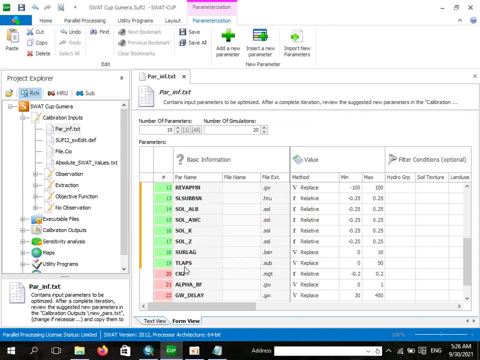 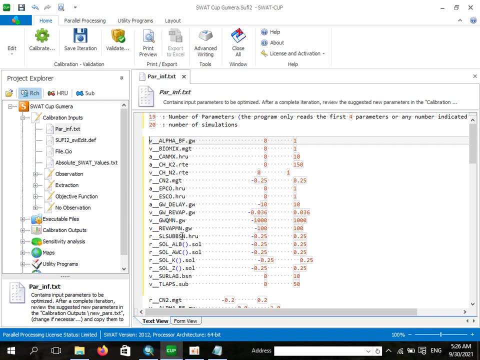 the number- yeah, here is the last number- is T labs. those highlighted in green are selected for this sensitivity analysis, while those reads rates are not selected for this analysis. so you can add your sensitive parameters in such a way you know that where, from where you are obtaining those parameters in the last video. so say, save it. 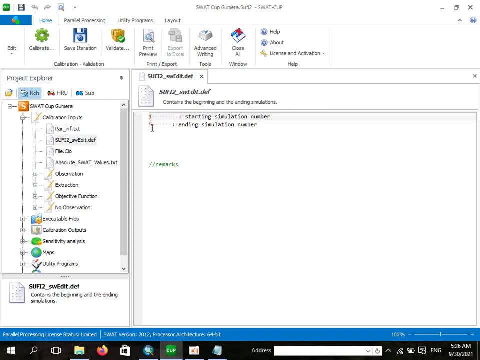 in the other series of feet. two: here is the starting simulation is number one in the ending simulation is out to T on you. I would like to see up to T on issuance simulations so you can edit in such a way and to say, save it and this file is. 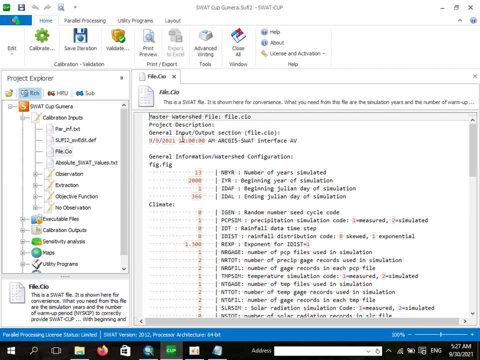 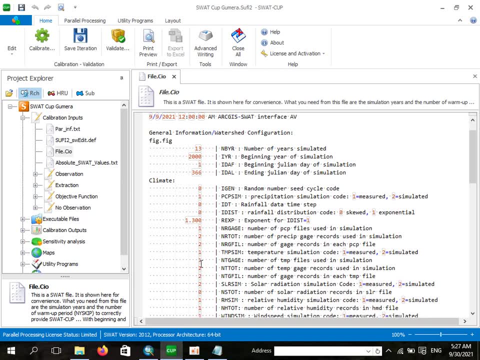 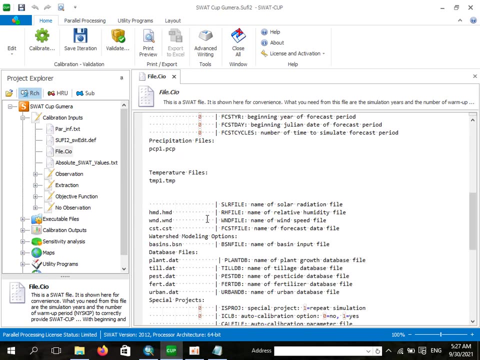 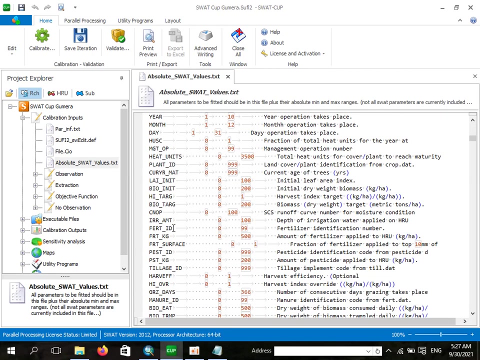 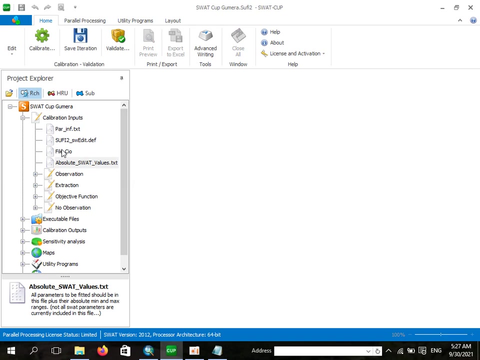 your eyes extracted from the swat, so you cannot. it is these things we can see. what are the yes, what are the inputs that the SWAT extractors- yeah, in this absolute SWAT- helps us to extract sensitive parameters or parameters for sensitivity analysis. therefore, we have finished the first parts of this one in. 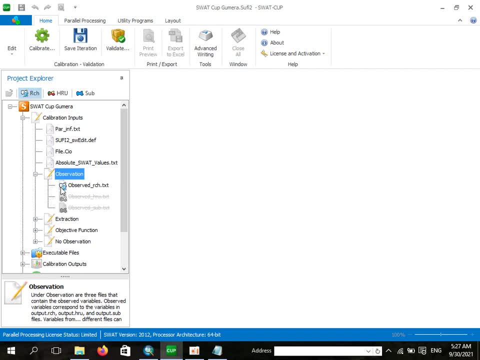 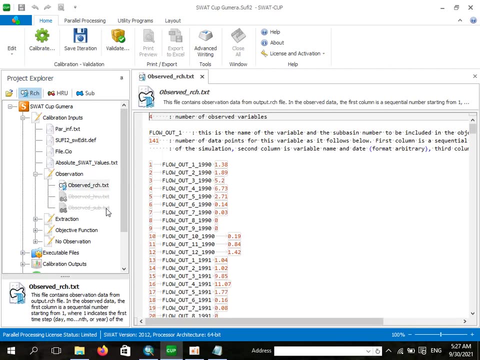 the second is, that is observation. since we have clicking this one, you should say that observer. it here is: I would like to observe one parameter which is a stream flow to the stream flow and you should edit in such a way that those parameters, those flow parameters, should be in such a way, that you should edit in such a way. 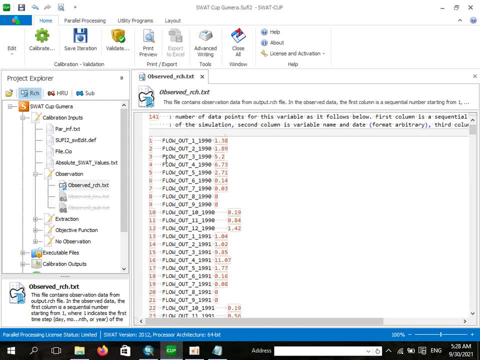 should be prepared in such a way. you see, this is that this SWAT cup needs your stream flow in such a way. there is a flow, there is flow out. when this is a monthly data, it puts in such a way the month and this is the year, this is a. 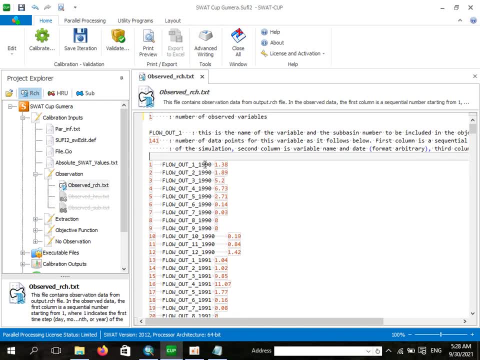 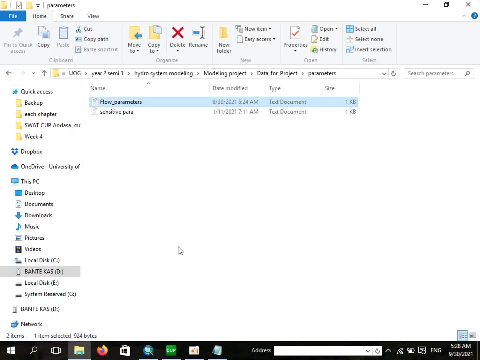 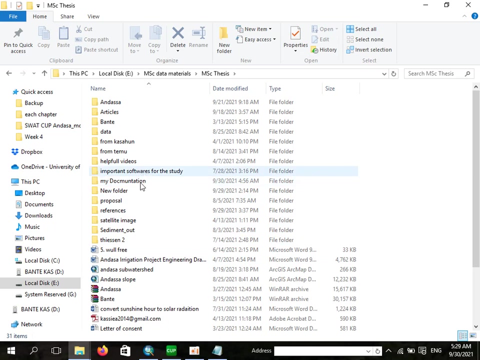 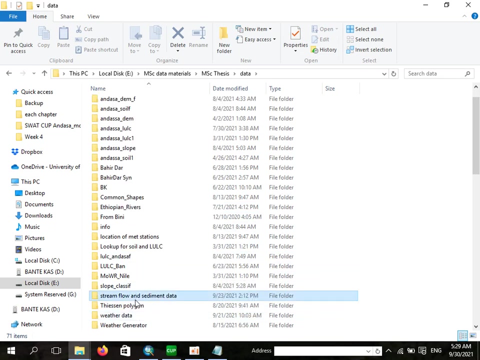 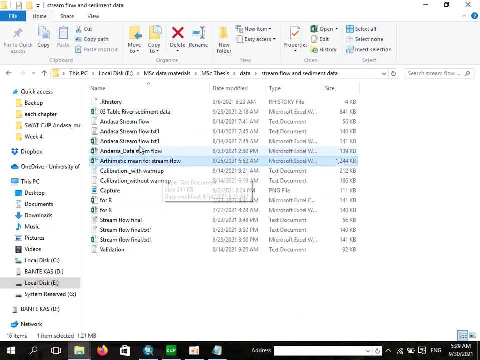 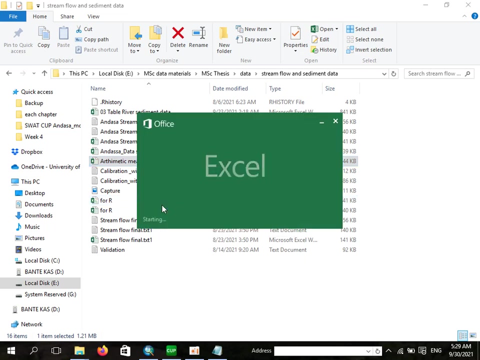 stream flow here, so you should adjust your stream flow. what's this? what cups are requiring? so let us first prepare this data, how to prepare this data for this illustration, and let me show you how you are preparing those status. okay, okay, those are these details, the details. okay, let me wait a minute. this exhale opens. let us 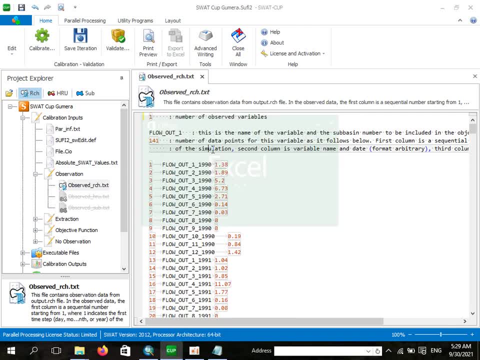 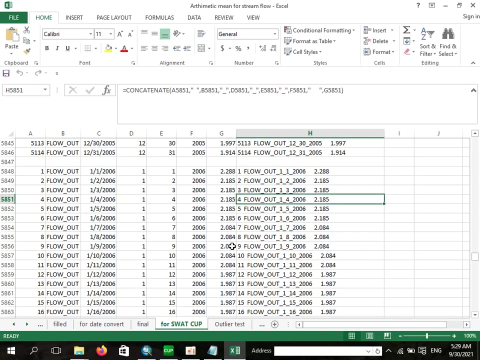 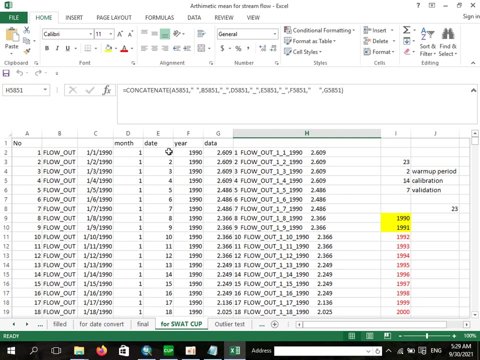 discuss one thing here. okay, so if we are obtaining or preparing our string flow in such a way, we will copy and paste under the section simply. therefore, that is very easy. so if you are, if you have, if you have and a fellow in such a way, for instance, if you. 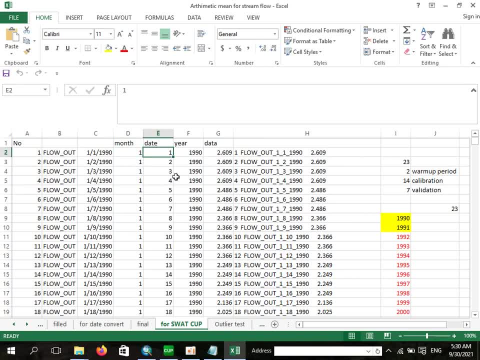 should have a man's here, a date here. if you are checking these in daily data, if you have daily data, provides you your case, because that is what I have to track, if you are? if you are, we can surely test it here. we can certainly level things, you can certainlylin. 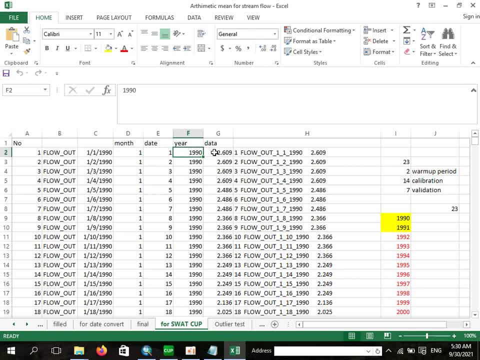 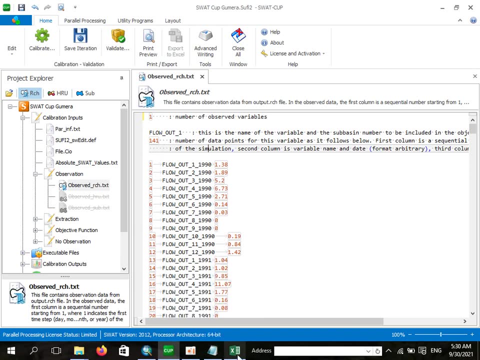 Well, if we have a low, like on low, our law, and if we are הי have a year here and you should have data in such a way, and also there is the numbers here, because you know that here is the numbers, so you should have this number and after that, if you have given, 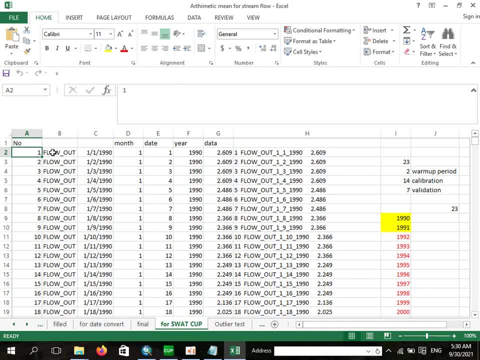 number for your data in such a way and when flow out, yeah, you should give, say in such a way: flow, underscore out, flow out and um. after you are preparing your data, you should do concatenating your data. okay, so concatenating that, your the equals concatenate number here. comma. 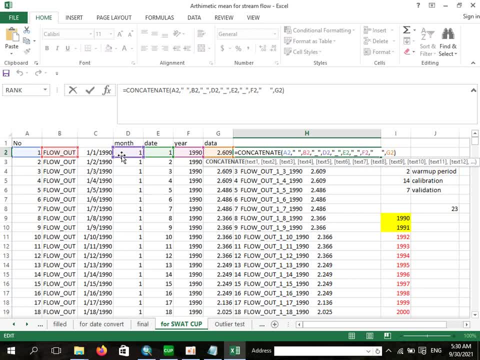 the flow out comma. the means here the date, the year and the data in such a way so, after you are saying enter, you can prepare a data in such a way so you can separate your data for calibration, validation as well as sensitivity analysis easily. as i have told you earlier, 10 percent of your data. 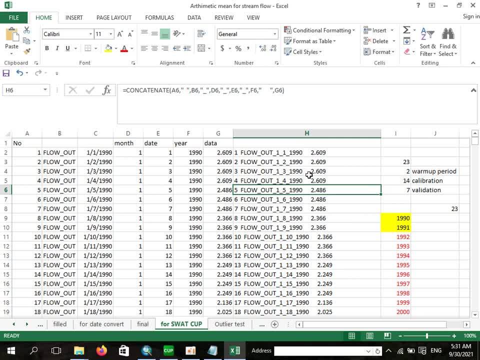 is used for using uh, used as a warm-up period, and the remaining from the remaining data. from the remaining data, two-thirds of your remaining data should be used for calibration, while one-third of your remaining data is for validation purpose, so you can prepare a data in such a way. okay, it. 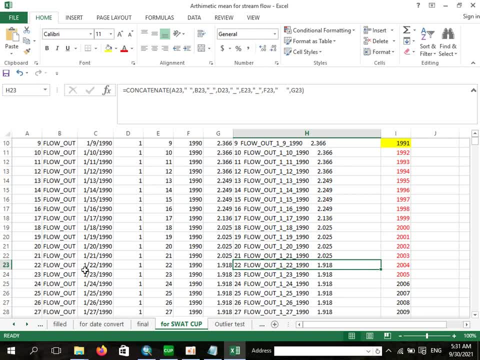 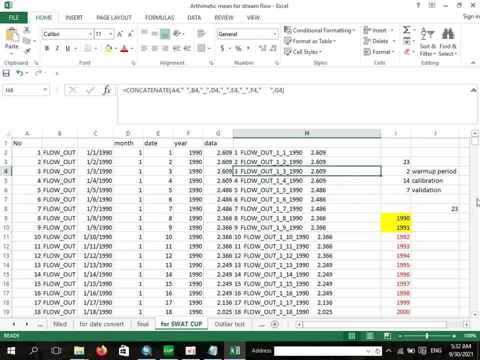 is very simple. you can exercise on your own. so after you have preparing it, you should prepare your data separately. separately, for instance, if you have, for instance, this date has a year of 23, so 10 percent of this one means 0.3, so two percent is. 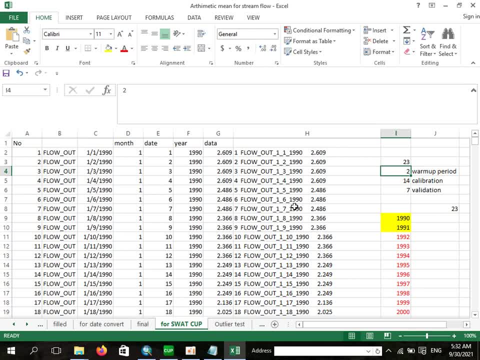 used as a warm-up period, and so to prepare your data for sensitivity, you should reduce two year data from the first years- maybe 1990 and 1991, as i used for warm-up period- so you can use the remaining years for your purpose and afterwards towards that for calibration. 40. 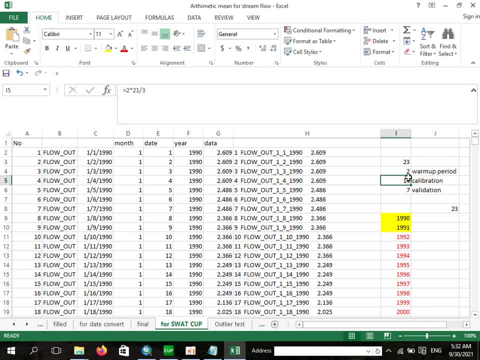 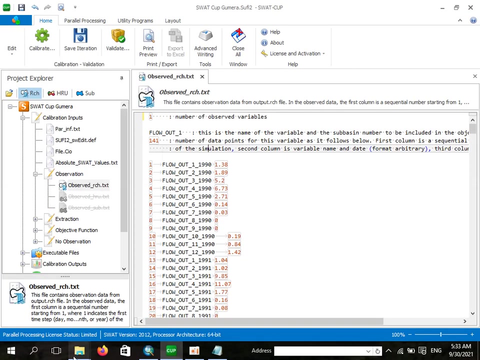 years. that means two thirds of you. any three minus two is 21, so two-thirds of 21 is 40 years. so you should use 40 years data for calibration in seven year data for validation purpose. so it is very simple. so let us see. let us see for the data, what we are preparing for this purpose. 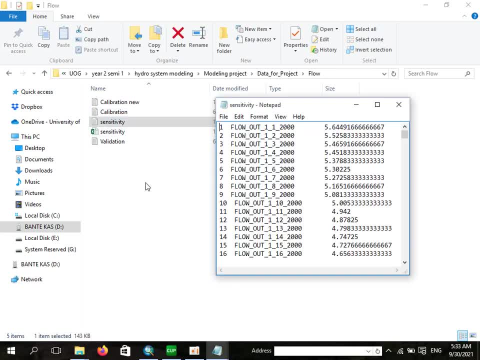 so let us ease, for sensitivity analysis is for sensitivity analysis, or latest are taken for sensitivity analysis from thousand up to 2009, but since this one is from 2000 to that of 2009 means 10 years data are used, so when one year for my period is. 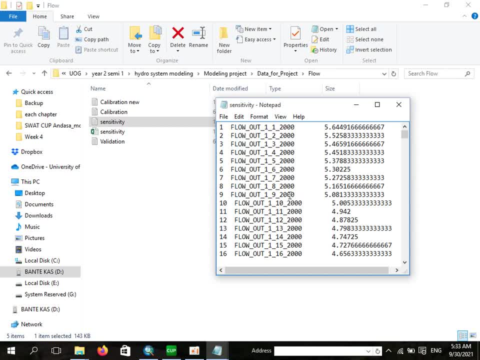 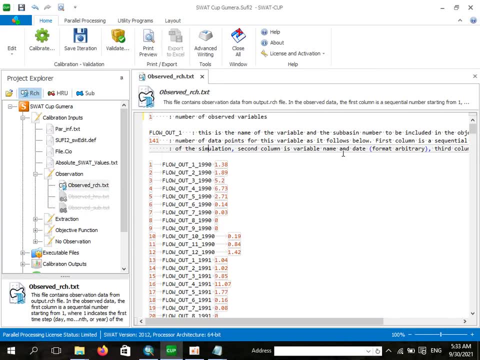 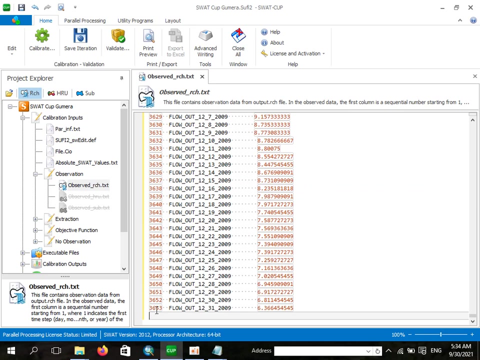 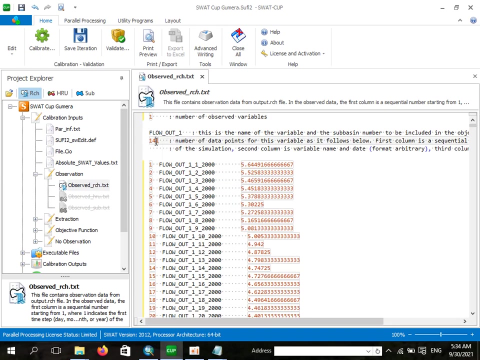 selected for this work so you can copy, select all copy, and since we are working for sensitivity analysis, you should use this one and just select this one and paste your data here. and the last number here is 36 53. 36, 36 53 is your data, the number of data. 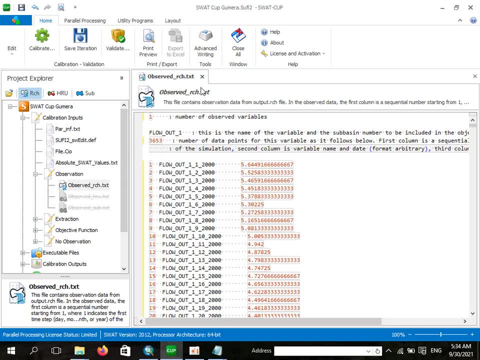 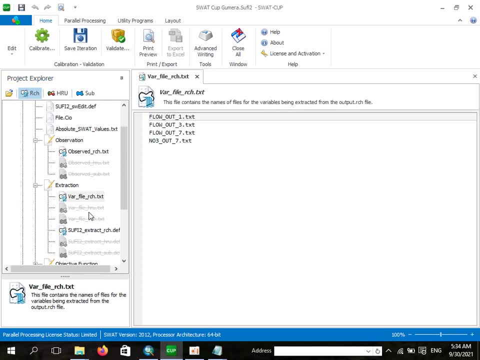 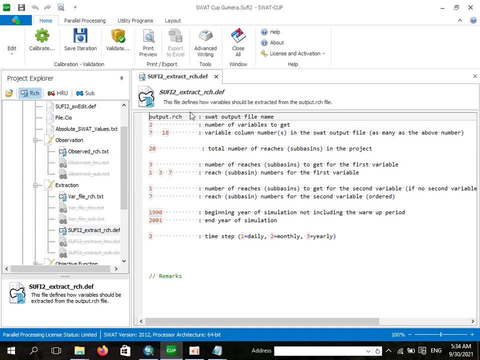 so you can adjust your data under observation in such a way, just save it, your data here, go to this extraction and under this variable file, i would like to know: only flow out when, flow out when and save your data in such a way, go to the sufi to extraction, or it's okay. so the number of variables to get is: 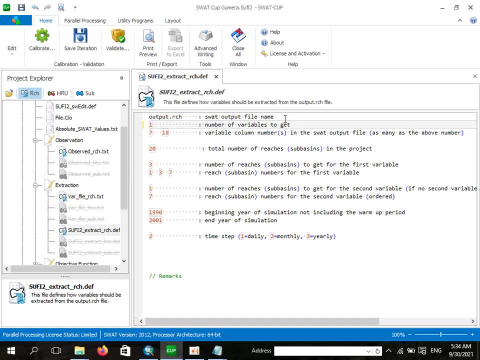 i would like to get one variable which is a stream flow, and this variable column number. in the output file this stream flow is located under seven, so you can give us seven. you can see this value from the outputs of your excel output, or that is what thousand. 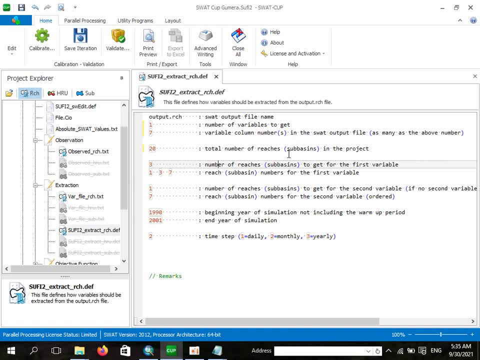 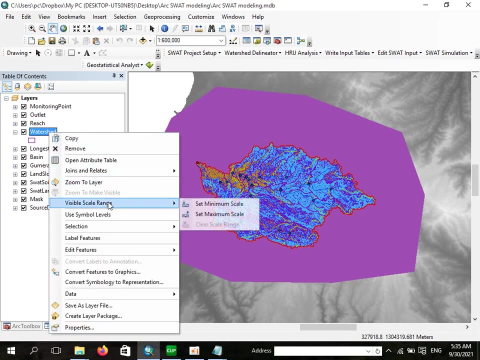 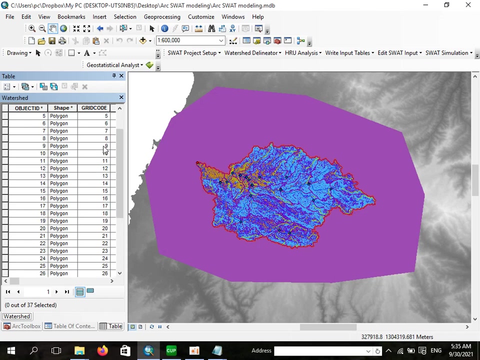 11 such a way the total number of fritz or as a business in the project. so to know that the total number of uh reaches you should go to your arcswath model here and open the attribute table here. so if you see here the total number of watersheds, total number of watersheds in this, 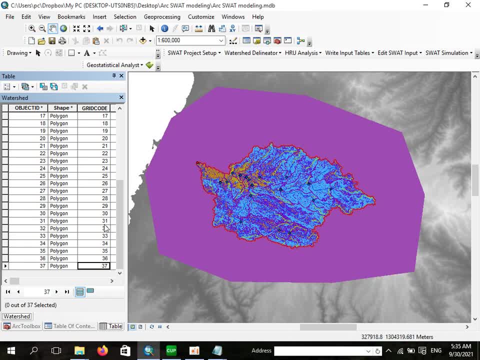 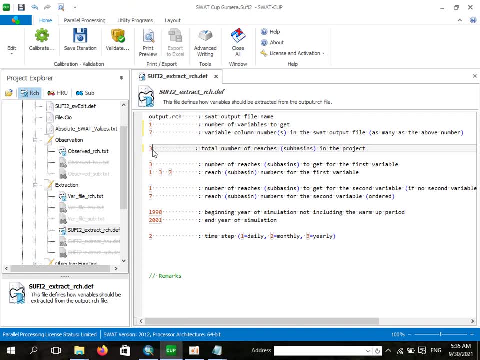 kumara watershed is 37, 37 sub watersheds, 37 sub watersheds, so you should read it- and 37 sub watersheds are here. number of reaches to give for the first variable is: similarly one, similarly one. that's the rich source, a busy number. for the first variable here is: you should take care here. 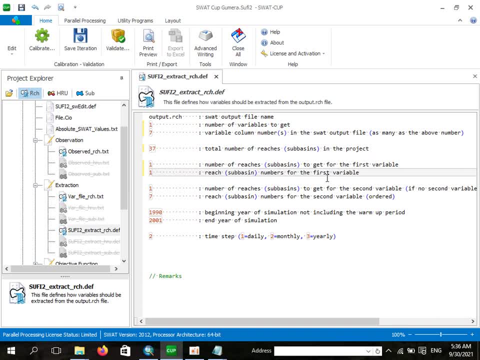 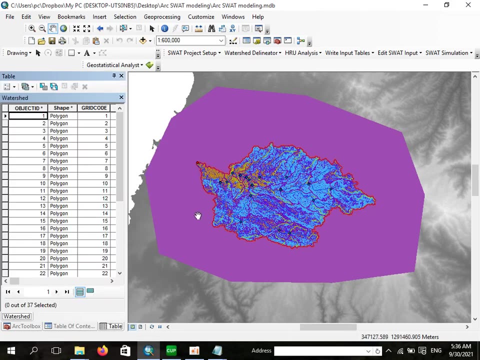 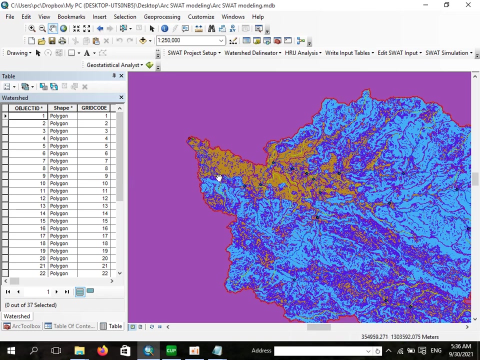 the first. the first number of variable means a rich number, for the first variable means that is, a number of sub watershed at the outlets of your watershed, for instance. if you open this one, open the attribute table and this means the number of the watershed. the numbers of watershed if we select this one is not included under this. 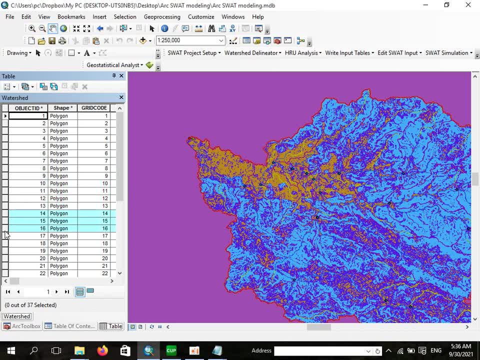 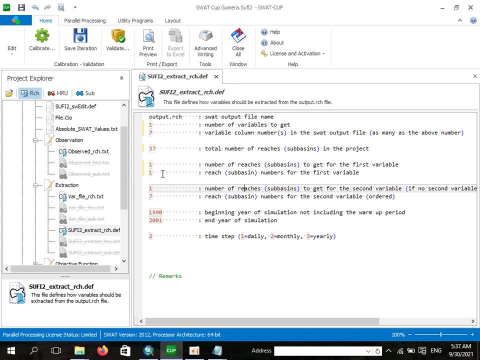 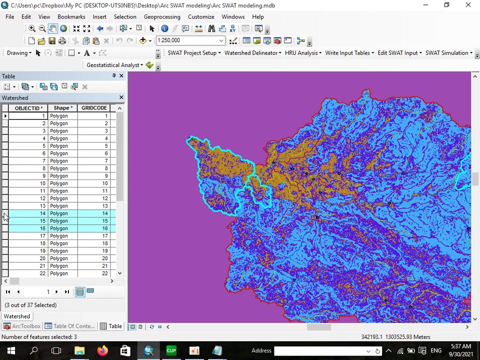 one. all right. okay, here is um this one, this sub watershed is the number of this watershed. that means the outlets of your watershed is occurring- is put in in this area. therefore, you should select simply this one. this number, 40, is the number of this sub watershed. that's the first variable is available, therefore. 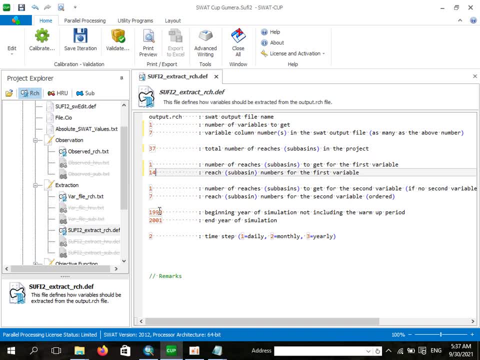 you should say one four, okay, one four, that's since we are working. uh, one variable, only, one variable only. you should delete this one. you should delete this part. okay, let us delete this. in the beginning here of simulation, not including the warmer period, is um not included in the warm-up period? 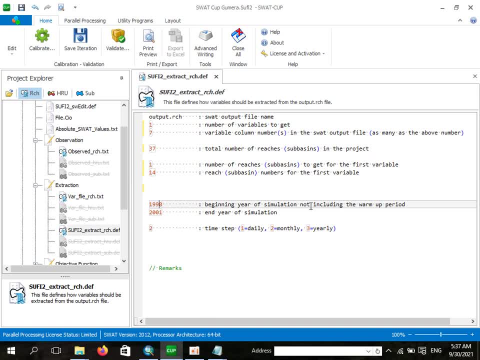 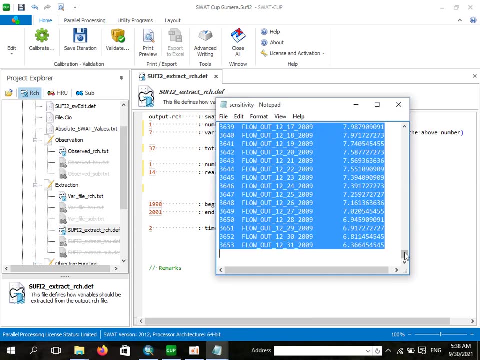 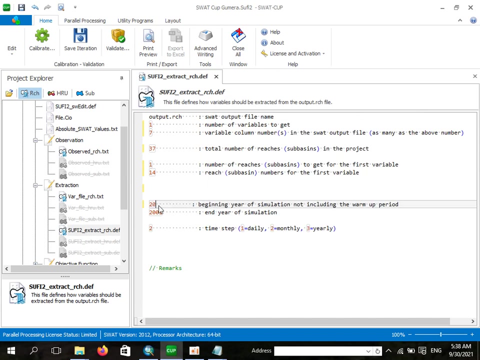 including the warm-up period. since we have 10 years streamflow data, you should take one year as warm-up period. so in the first year of the first year, here is: the first year is 2000, so you should give us here is 2001 and it in this uh to 2009. 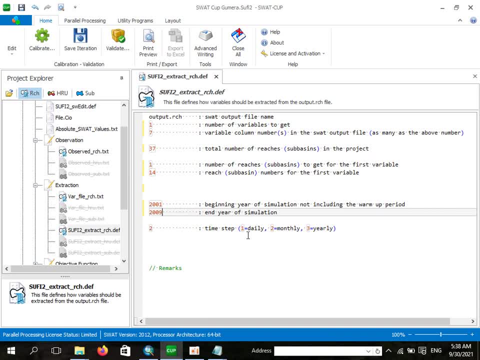 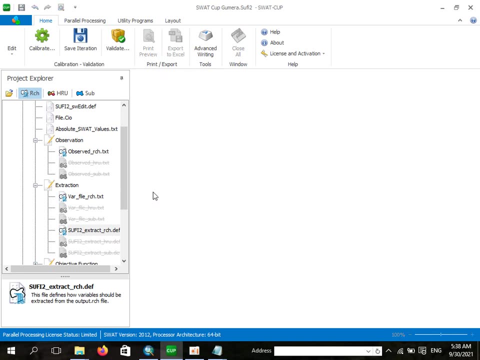 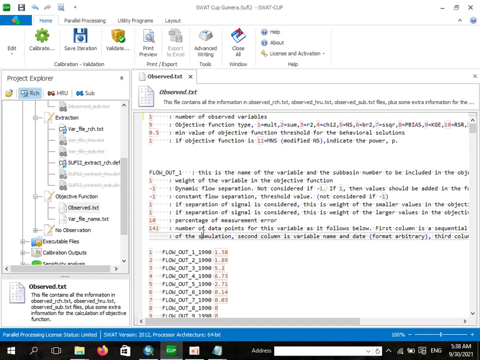 and i would like to select the time step as daily time step, daily time step in such a way. therefore, i have finished this editing this extraction data and say yes, save it. and subjective function- here is objective function- is observed. this one is when- here is when, and you should select all the datas here. similarly, those datas copy and: 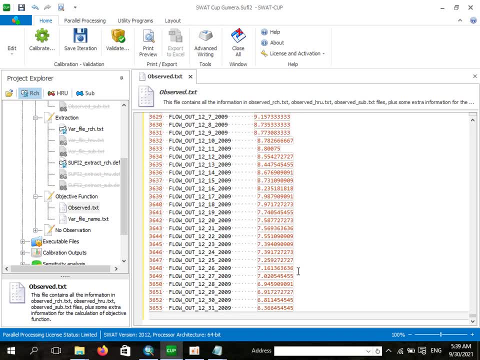 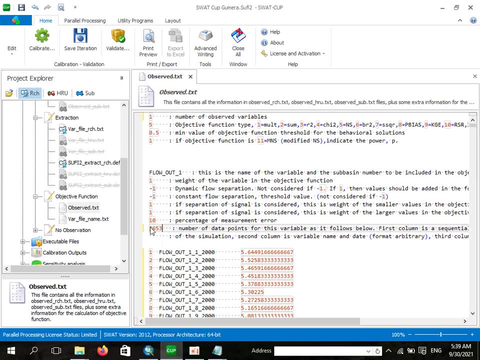 select in such a way, paste your data: 36 53, 36 53. 36 53 is a total data and you know we have already finished, as other things are not. uh, let us tell you something. here is five objective function and, basically, when we are doing, the performance of our model. uh, for hydrological models, this nice. 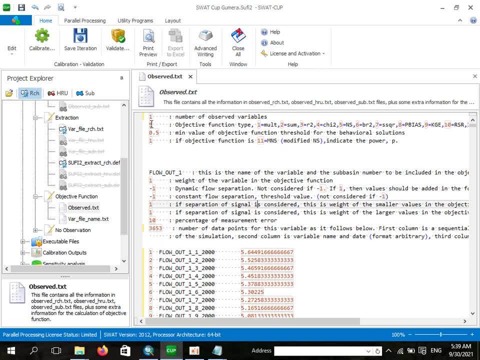 is most advisable. so that's why, uh, these five indicates okay, i would like to show the nice article efficiency. so, unless you can use another parameter like r square, but this nice article efficiency is mostly advisable unless we lost this pbs, percent opiates, that means is also advisable, so you can select some parameter. okay, software that you can save your. 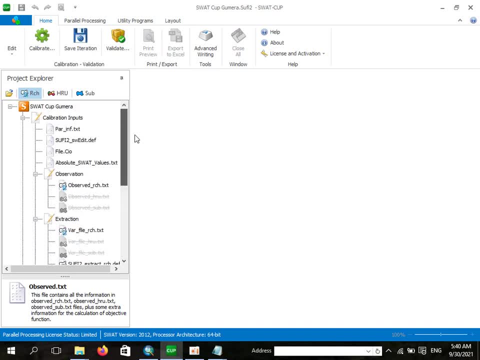 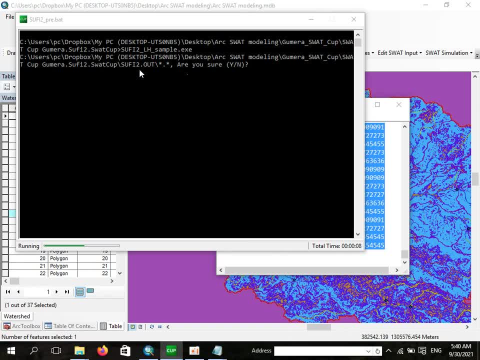 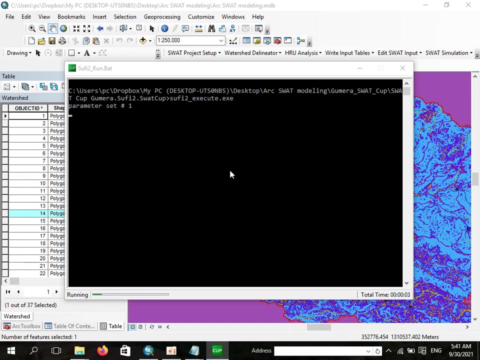 and it says: if you are, if you are in terms to continue, and just, you can write as well that if you are considering you as a meeting, a mistake, you can click and now, by writing in, so say enter, yes, okay, okay, start the execution. you see, uh, those are these swat cap are. 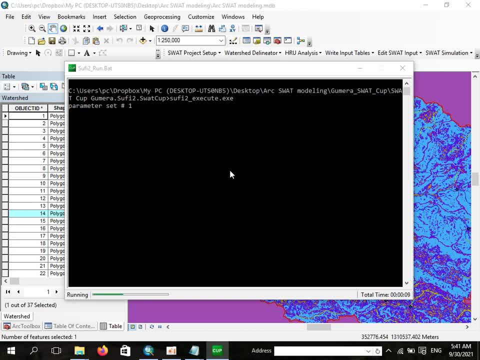 starting uh to work for sensitivity analysis, so i hope this is very simple and you can handle the sensitivity analysis using swat. cap means what's the cup 2019 in such a way. so, since it takes a lot of time, it is better to pause and we will see as a result of our work. 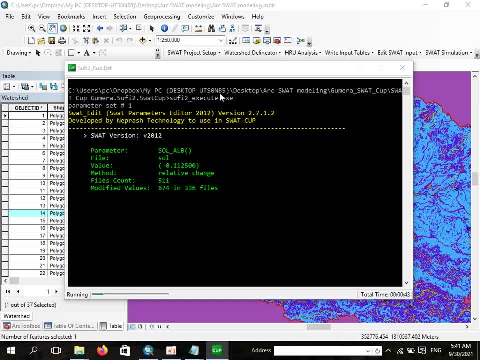 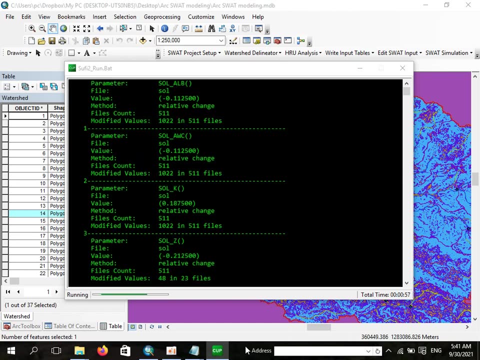 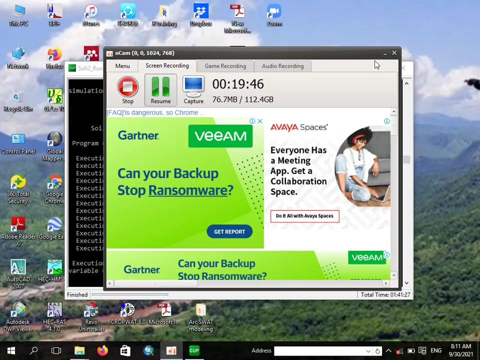 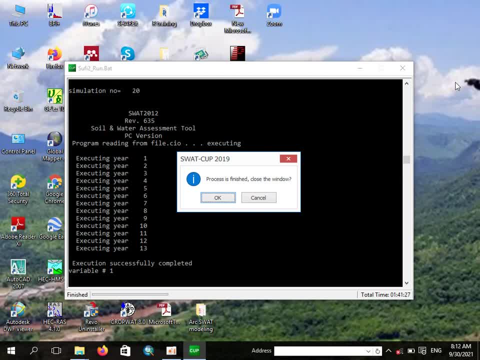 okay, so, uh, the sensitivity analysis is, uh, the sensitivity analysis is, uh, the sensitivity analysis is, uh, now finished, as you see here. now finished, as you see here, now finished, as you see here. uh, as you have seen, uh, as you have seen, uh, as you have seen, we have